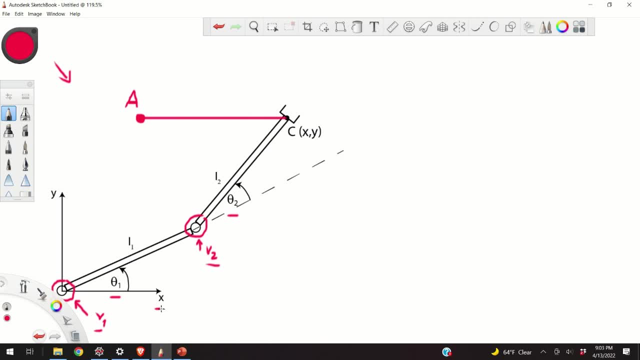 however, the control problem is usually expressed in the world or in the cartesian coordinates, and our assignment is to move this point c, or the tool center point, from some initial condition to the final condition, and in this case, i have to follow a straight line. now, since you are only controlling, 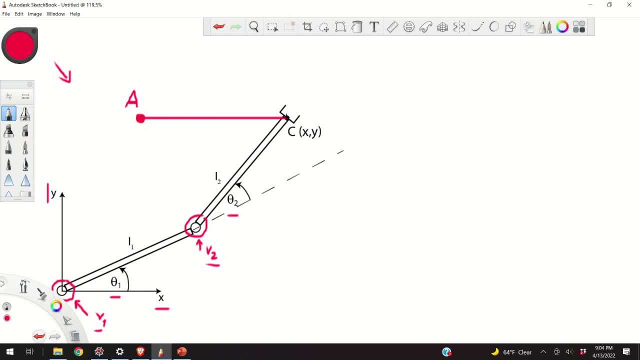 theta 1 and theta 2. you're not directly controlling the tcp, the tool center point. you need to. for a given final destination point, for given coordinates of the final destination points, let's say coordinates xa and ya, you need to find the corresponding angles of rotations. let's say theta 1a. 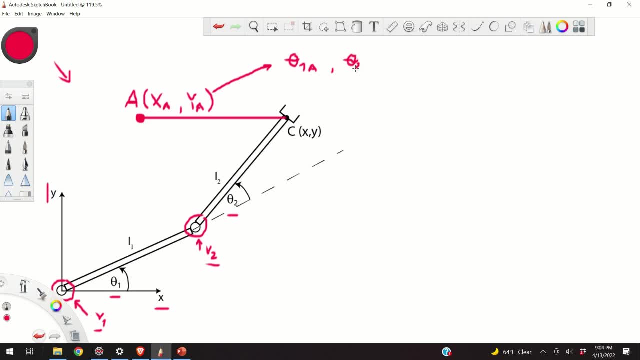 and theta 2a. that will bring my point c to this point, so you can think of situation where your robotic manipulator will be in this position, for example. i'm now exaggerating in order to illustrate you the basic principle here. in this particular example, my theta 2a will be this thing: 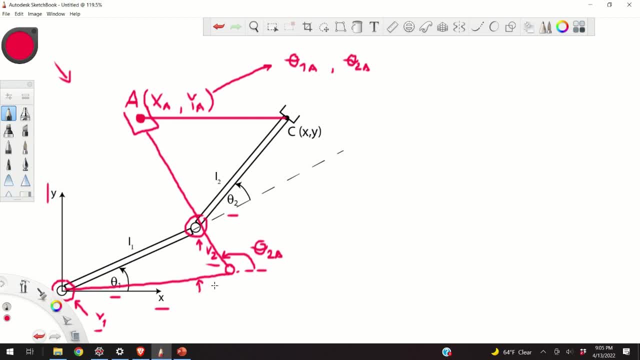 and my theta 1a will be this thing over here. so if i specify that were the TM here I am going to find those religious animal moments which are killed with force by tcp. so if this happens, the new Boolean Darwinsonaro�� Doc das. you might ever imagine that have processes for mannequing large the holidays step to buriers. say why a I need to find how I need to control my motors in internal points, that is, given the external coordinates. these are the external coordinates. said why a I need to find how I need to control my motors: internal coordinates such that my manipulator will be in force with an external. 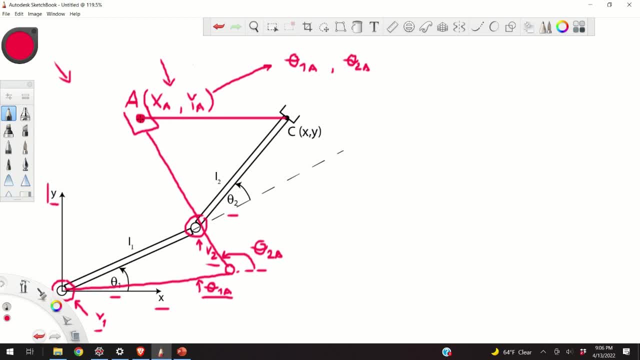 ends at this position, That is, its TCP tool center point goes to the position A And, roughly speaking, that's the inverse kinematics problem. In reality, you're not going to have only one point, you're going to have a bunch of points along this straight line. 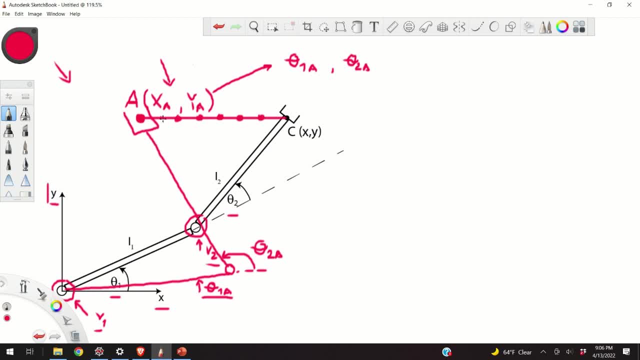 that describes the trajectory of my point C. So you will first have to interpolate this line and to find a bunch of points, And for each of these points you will need to solve the inverse kinematics problem. Okay, So let us go to our original picture. 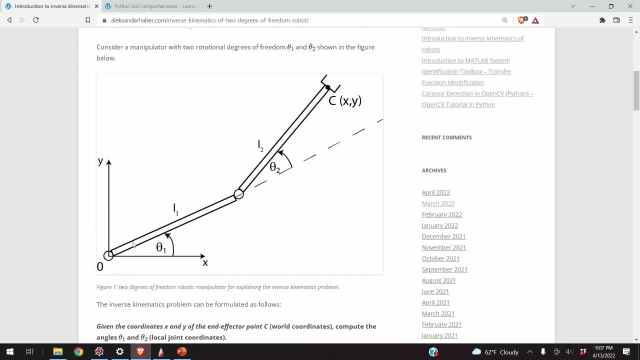 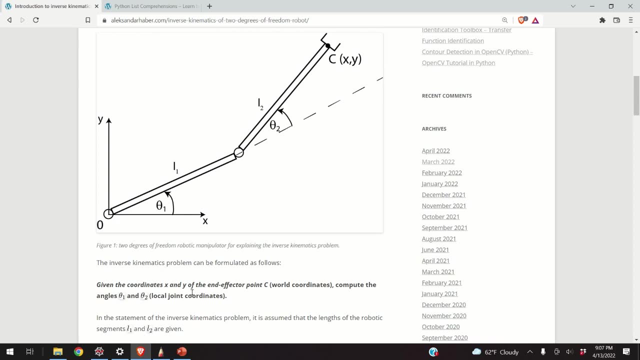 Here I will assume that this is the final destination point, That is, the C is in the final destination point And for this point, for this position basically, or for this pose, the inverse kinematics problem can be defined as follows: 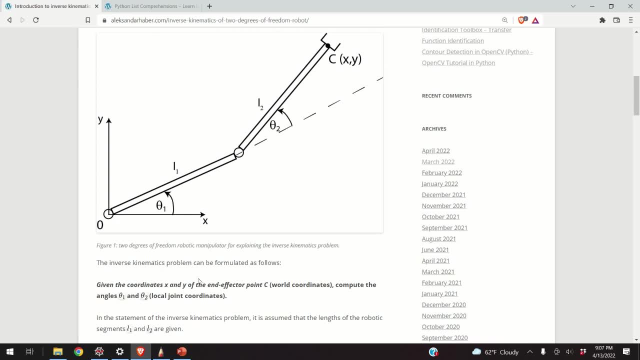 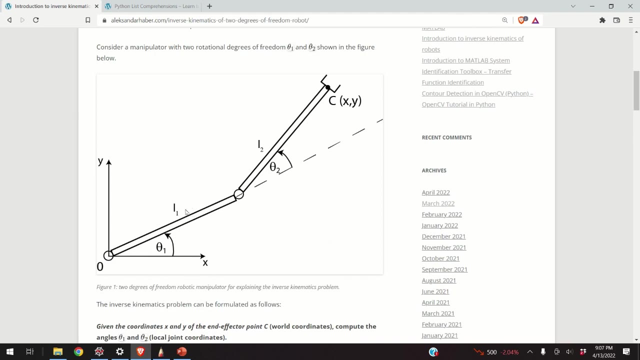 So, given the coordinates X and Y of the end-effector, point C, that is in the world coordinates, compute the angles θ1 and θ2.. Now, obviously, in the statement of the inverse kinematics problem, it's assumed that the lengths of the segment are given. 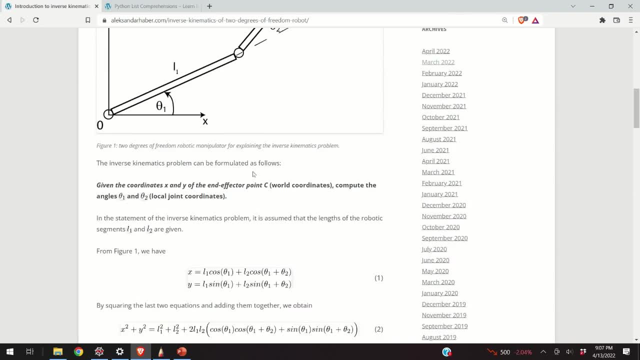 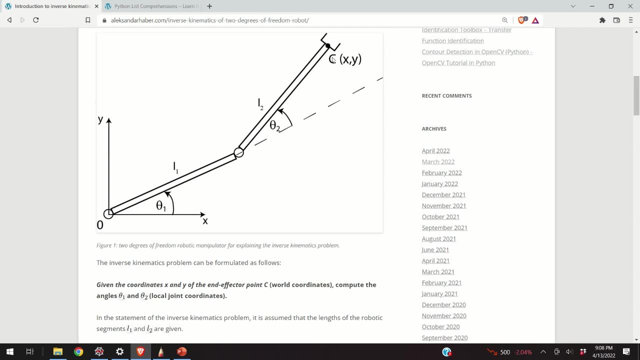 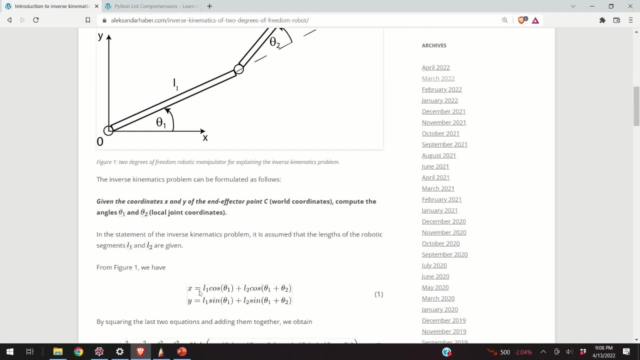 So L1 and L2 are given. So from basic trigonometry we can express the position of the point C in the X and Y world coordinates as follows: X is L1- cosθ1, so L1- cosθ1,. 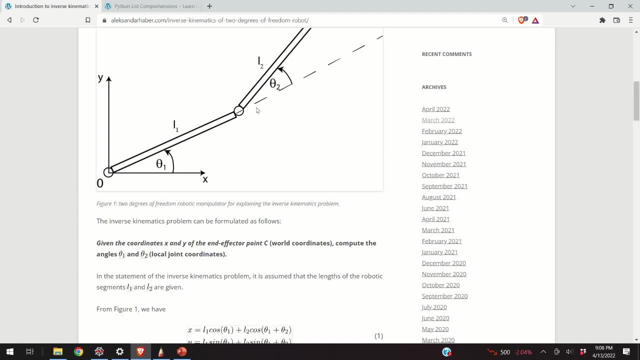 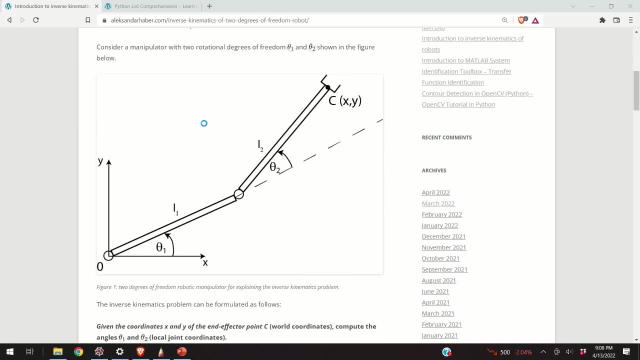 plus L2, cosθ1 plus θ2, right. So if you basically analyze this graph- I'm bringing now my epic pen- you will see something like this. So this part over here from this triangle is what? 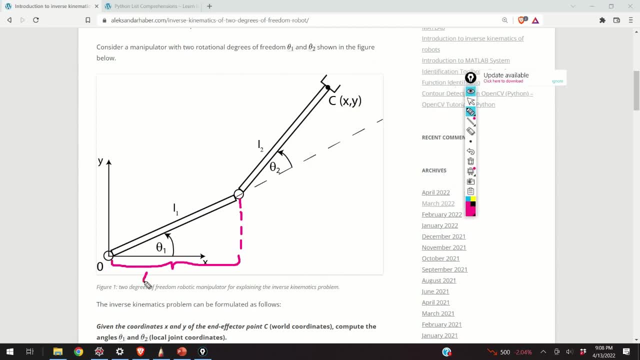 Is basically L1- cosθ1.. And this part over here- let me just draw a vertical line- is nothing less than the part over here, And the part over here is obviously L2, cosθ1 plus θ2.. And here I will just erase this. 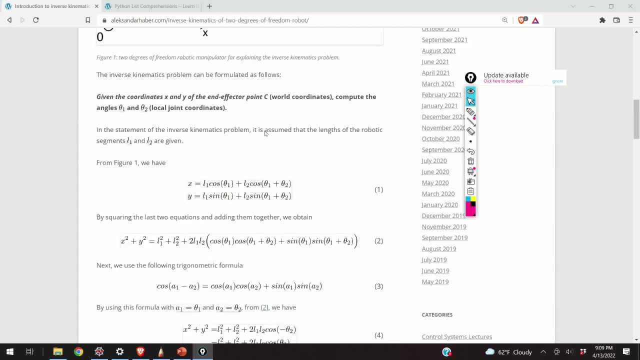 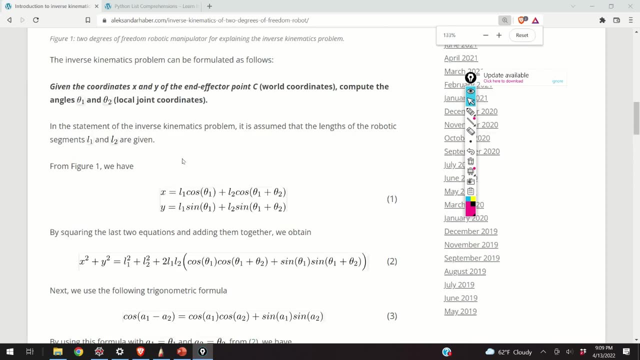 since I don't want to destroy my nice picture. Okay, so we have that X is equal to this and Y is equal to this, And from this equation we basically need to find θ1 and θ2.. From the mathematical point of view, 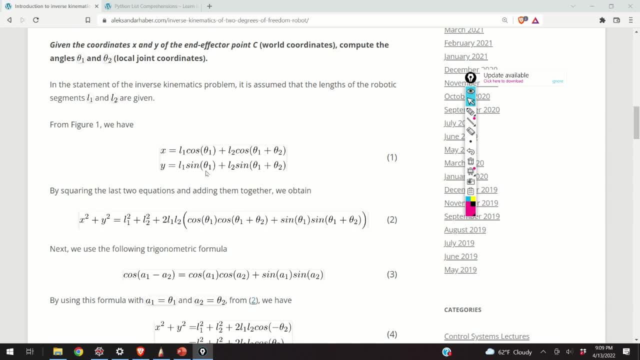 this represents the system of two equations with two unknowns. Unknowns are θ1 and θ2.. Knowns are X, L1, and θ2.. Knowns are L1, L2,, Y, L1, and L2.. 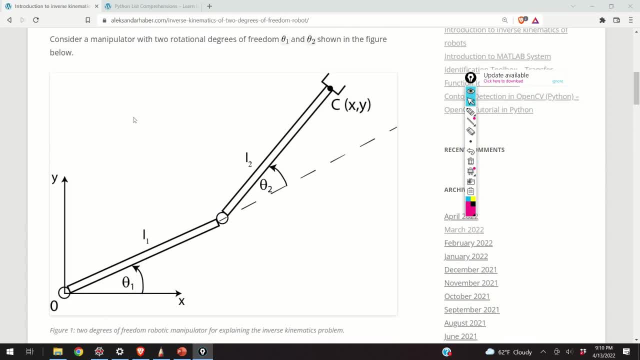 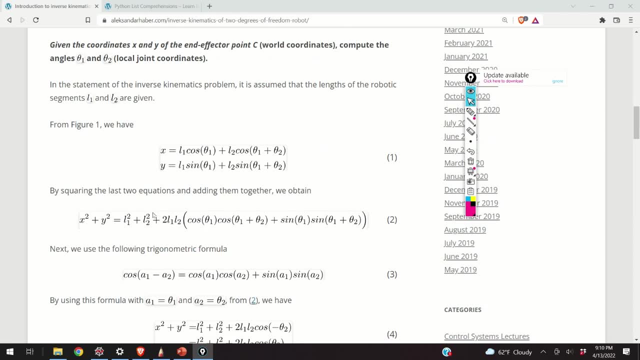 So, given any position, for example the position over here, I can define the system and I need to find θ1 and θ2.. So let us find θ1 and θ2.. Now, if we square this equation, 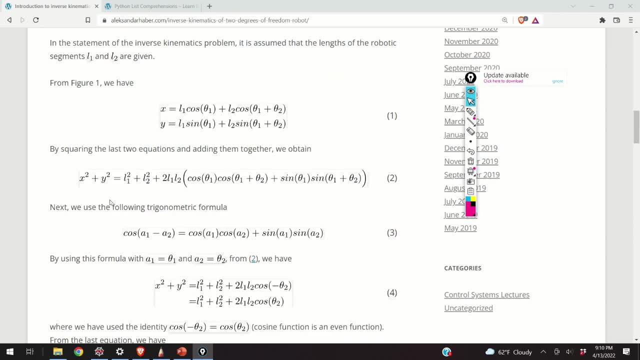 and if we add to the square of the second equation, we obtain something like this: Right Now, here you will see basically that this part over here can be simplified by using this formula: So cos of some arbitrary angles: a1 and a minus a2,. 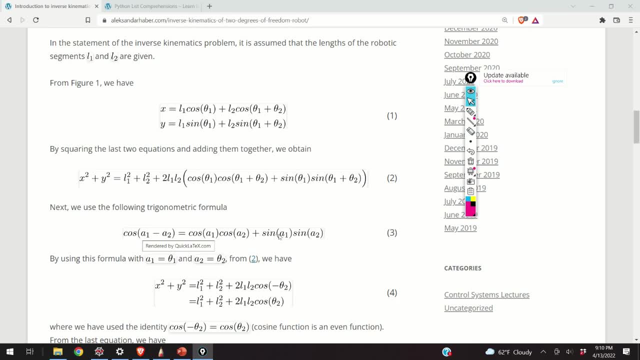 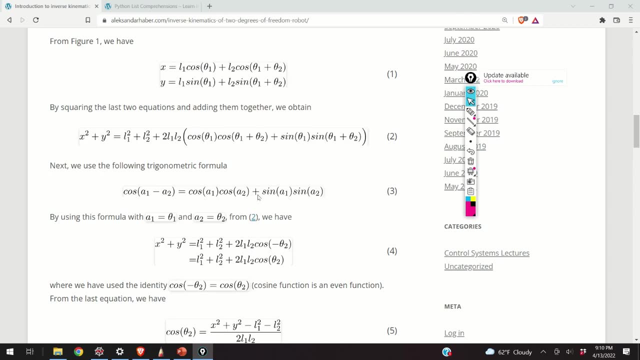 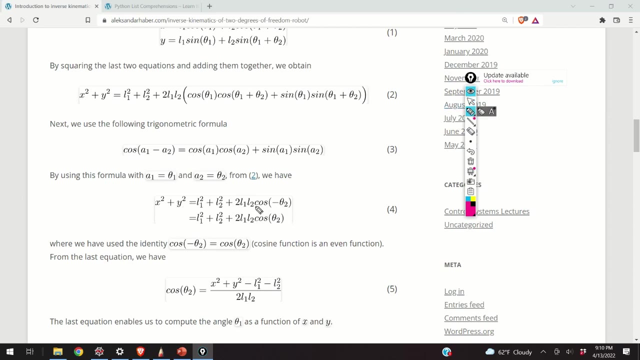 is equal to cos, cos plus sin, sin. Now if we use this trigonometric function or trigonometric identity and we substitute over here, we will obtain this equation. Now, here you should be kept in mind that the cos 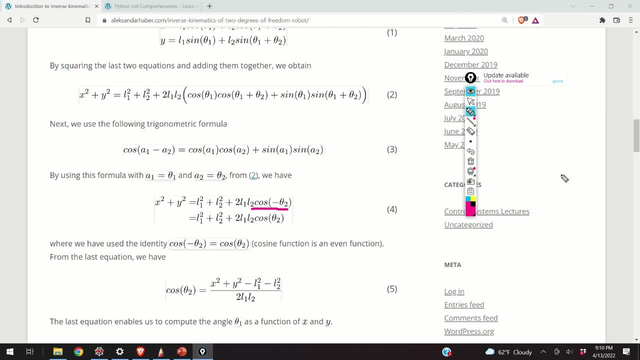 is an even function. What does it mean? So if this is your unit circle here, if this angle is θ, the cos is equal to this part over here. Let's just change the color. So this is the cos. 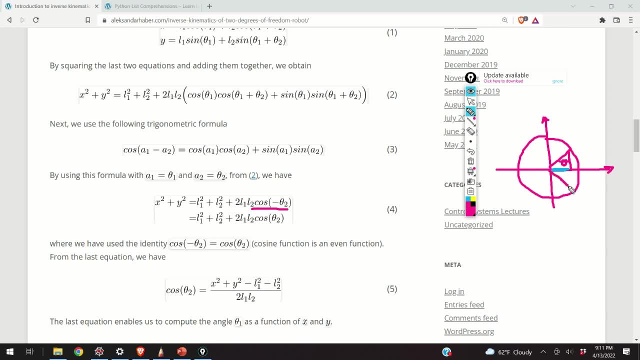 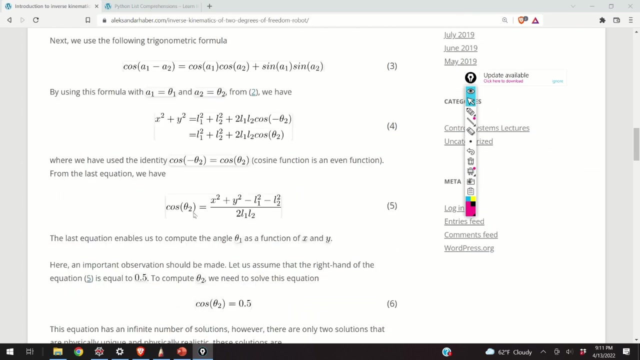 Now this cos is obviously equal to the cos. So if this angle is here minus θ, the cos stays the same. So cos is equal to cos. Let us erase this and continue Now. from this equation, obviously we can express the cos. 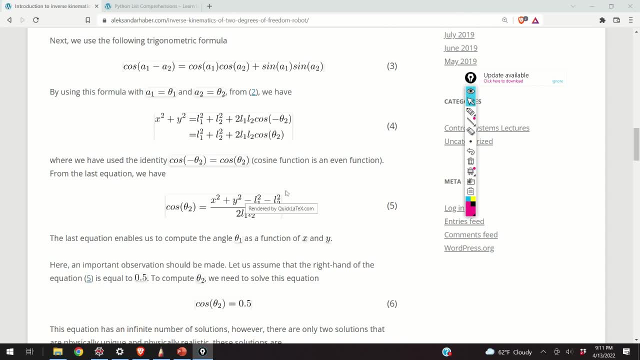 and everything that goes on the right-hand side is known: x² plus y², minus l1², minus l2², divided by 2l1l2.. So this is perfectly known. Okay, Now the question is: how many solutions? 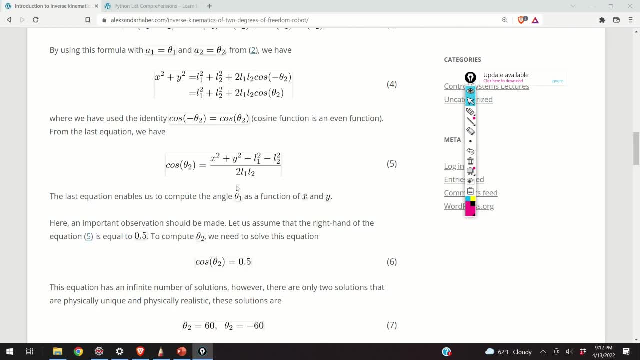 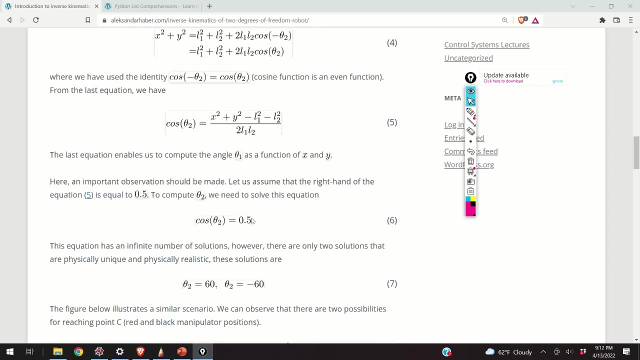 do we have over here? Do we have one solution, two solutions, three solutions, five solutions, hundred or infinite number of solutions? For example, let us assume that this side is equal to 0.5.. Okay, So we know that. 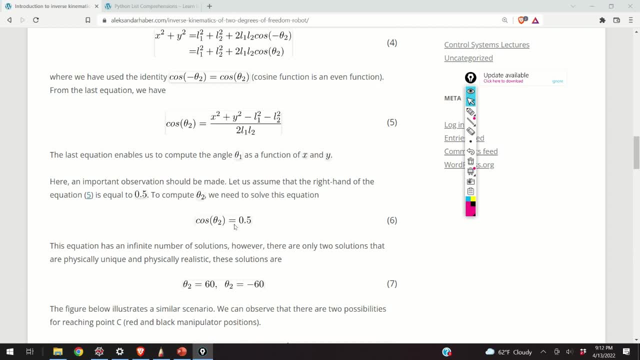 basically, if cos of an angle is equal to 0.5, then θ will be equal to 60 degrees or minus 60 degrees. Well, I said something that is not correct. Why? Because we know from a mathematical point of view. 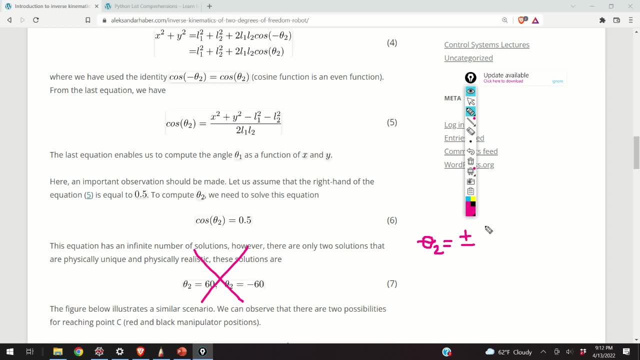 that the solutions can be expressed as follows: Okay, So we have actually an infinite number of solutions where this k is just an iterator. It can be 0,, 1,, 2, until infinity. So we in practice, 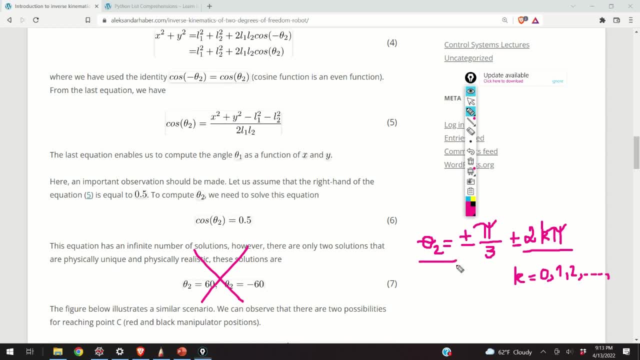 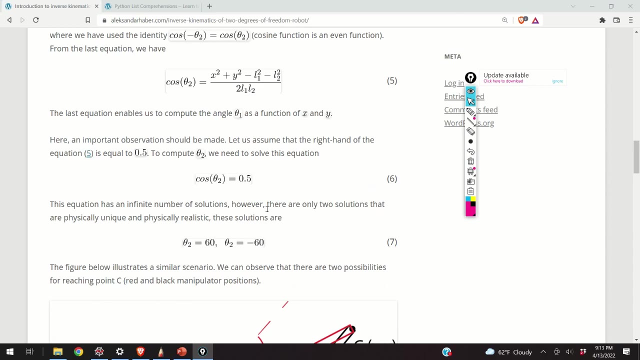 actually, from a mathematical point of view, we have an infinite number of solutions. However, there are only two solutions that are physically achievable. These solutions are 60 degrees and minus 60 degrees. Now, by doing this simple example, I illustrated you the first. 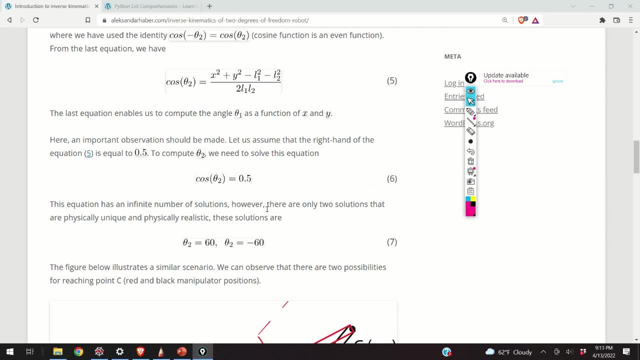 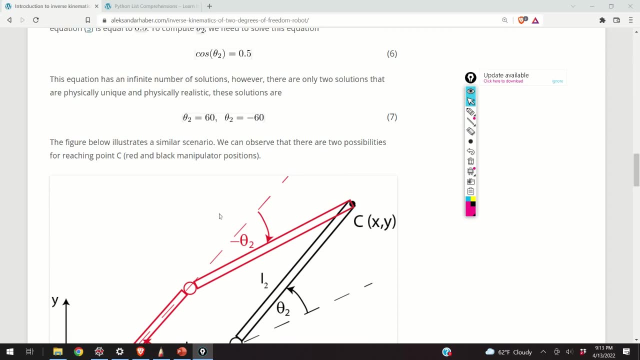 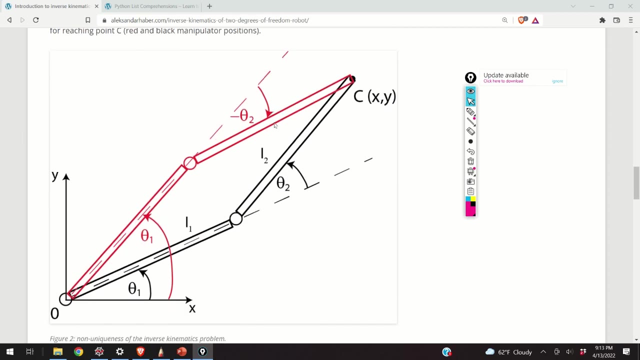 difficulty with the inverse kinematics problem. So the first issue with the inverse kinematics problem is that you have many solutions. It's not uniquely solved. You cannot uniquely solve it. Maybe some special cases, yes. So what happens in practice? 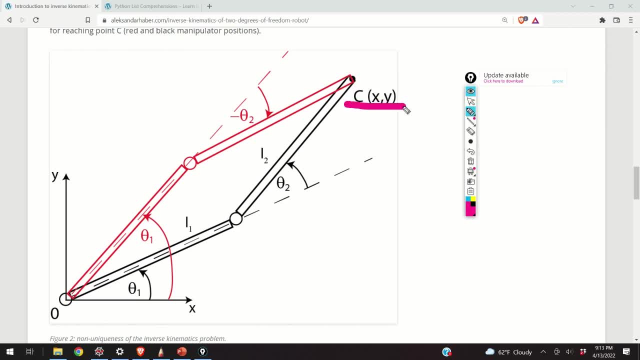 Well, we can reach this point over here in two possible ways. The first way, obviously, is this way right, And the second way is illustrated over here. So this is the second way for reaching this point. In the first case, 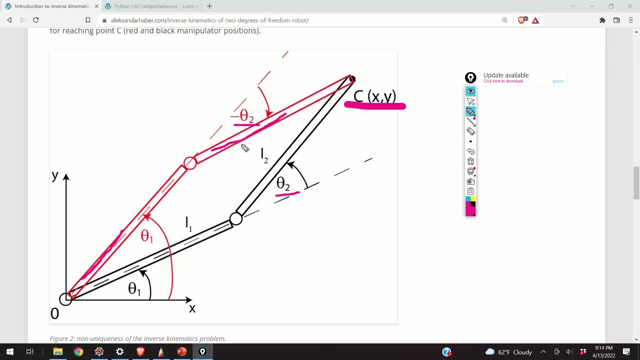 theta 2 will be positive and in the second case it will be negative, Because we always measure theta 2 starting from the direction of the previous link. That's the convention, And obviously the solution of theta 2 will influence the solution of theta 1.. 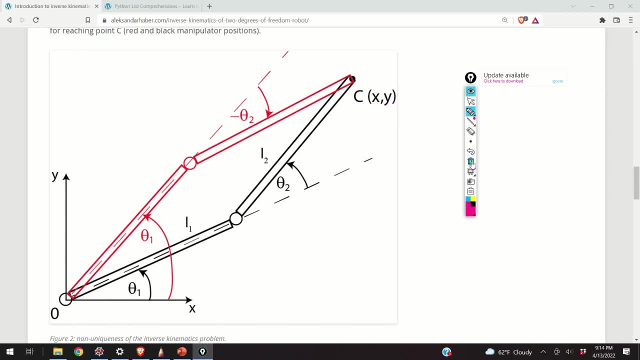 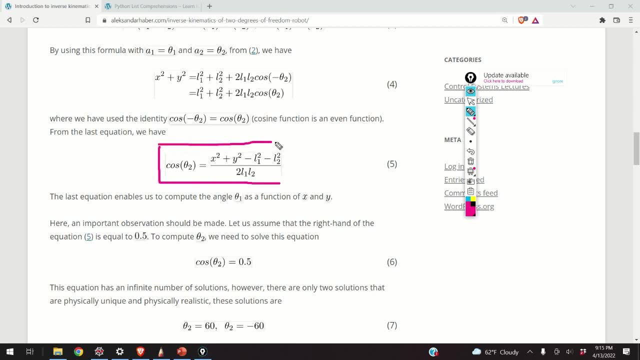 And you will see that later. Now, to summarize, this equation gives us theta 2.. So for any value of x and y, l1, l2, l1, and l2 that is physically achievable, we can find theta 2.. 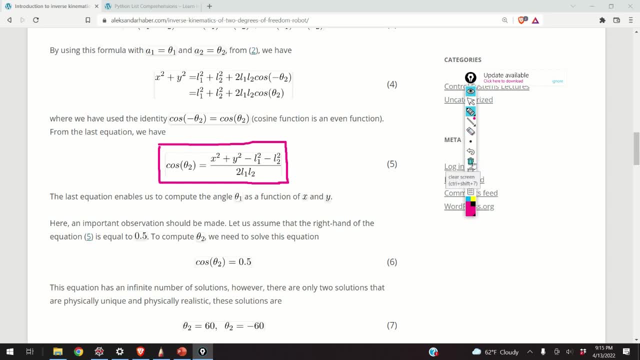 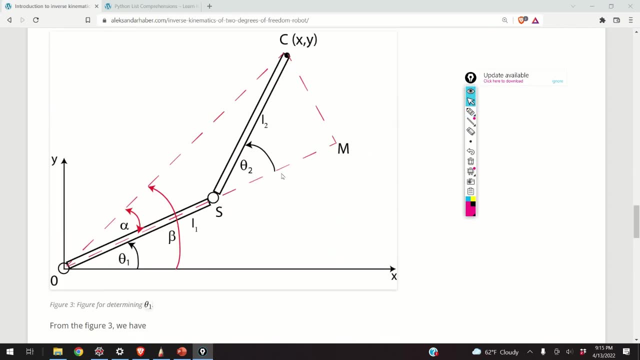 And we know that the solution is not unique. Okay, So let us find now theta 1.. So how to find the theta 1?? To find theta 1, we need to define two additional angles. We define this angle beta. 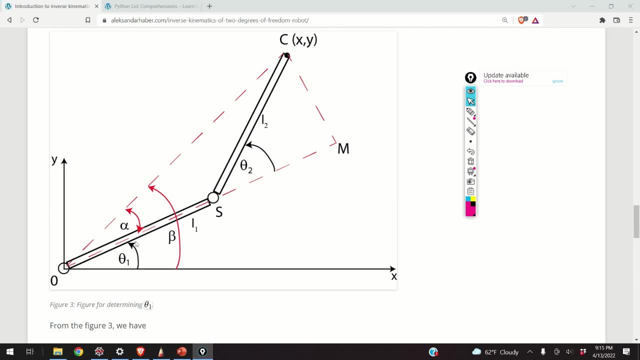 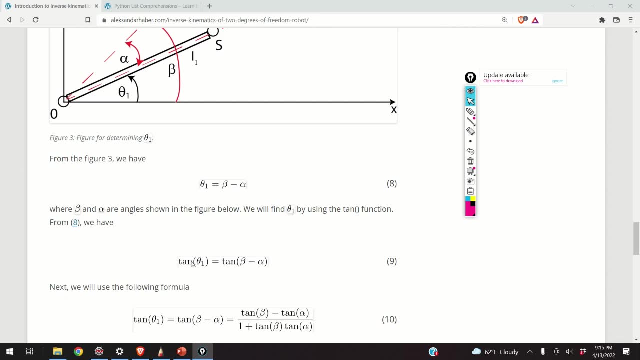 and we define this angle alpha. So theta 1 will be beta minus alpha And we will use the tangents Tangents of theta 1.. So tangents of theta 1 is equal to tangents of beta minus alpha. 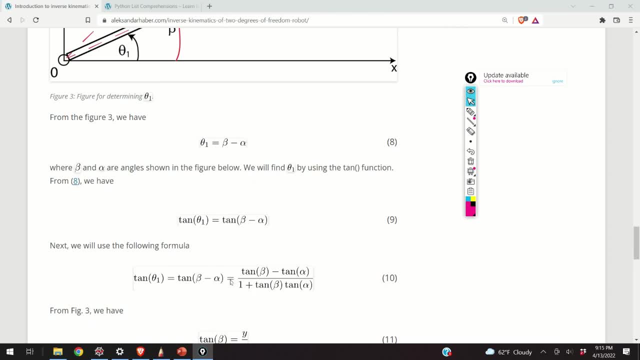 And we can express tangents of beta minus alpha using this trigonometric identity. So we can say: tangents of beta minus alpha is tangents of beta minus tangents alpha. 1 plus tangents of beta is tangents of alpha. 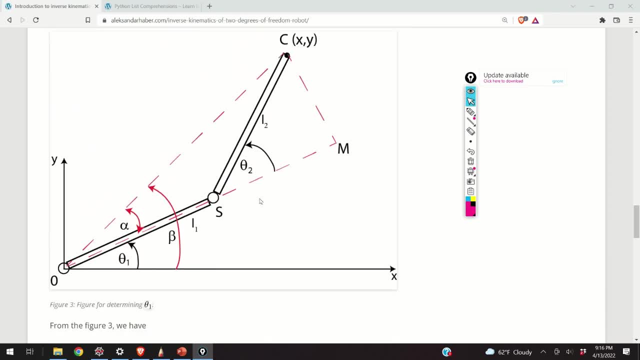 And we know that tangents of beta is y over x. So, looking from this triangle, here is the angle beta, Here are the values, right, This will be the y coordinate and this will be the x coordinate. So, tangents of beta. 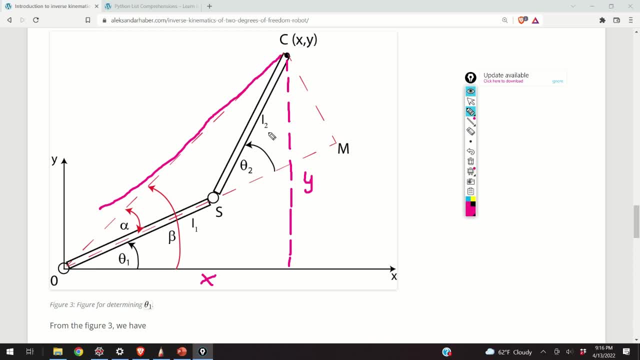 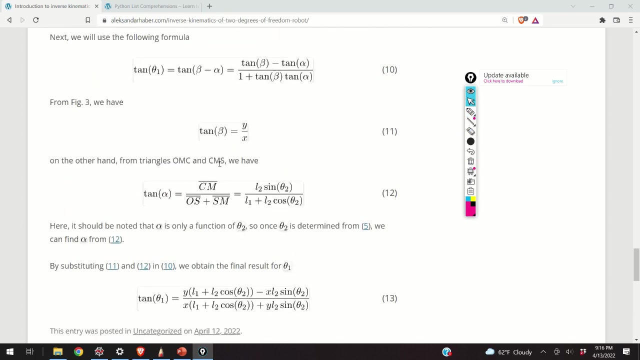 from this triangle over here. Okay, Let me erase this. So from the triangle that you can see over here, we can find basically that tangents of beta is y over x. Okay, So we know that that's correct. Now let's see what is tangents of alpha equal to. 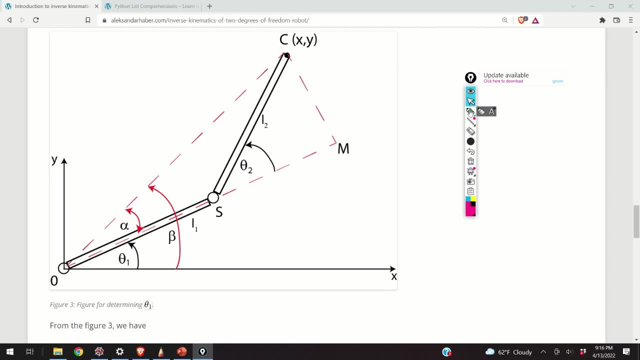 Now, looking again, tangents of alpha from this triangle. the triangle that you can see over here is equal to this side, over this side, This side. So this side is cm and the other side is om, So we have cm over om. 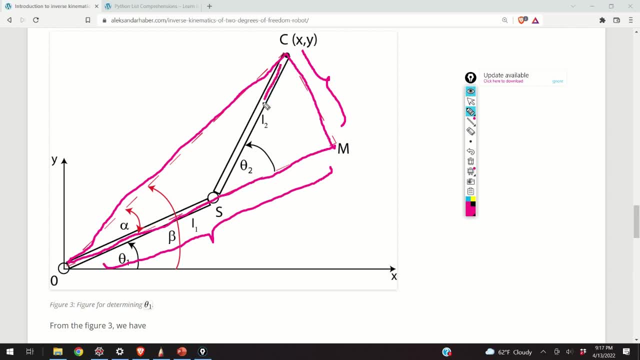 Obviously from this triangle over here, or let me use another color to better explain you. So from this triangle that you can see over here. what do we see? We see the following: We see basically that tangents theta 2 is this over this. 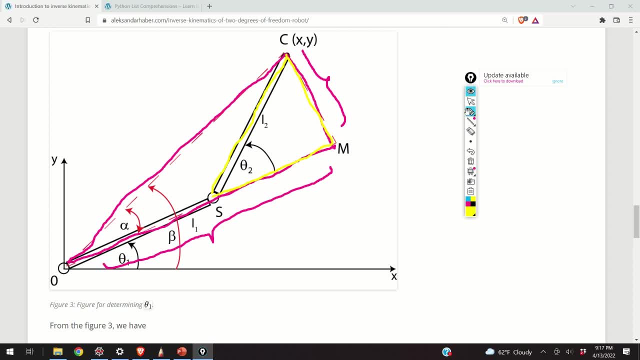 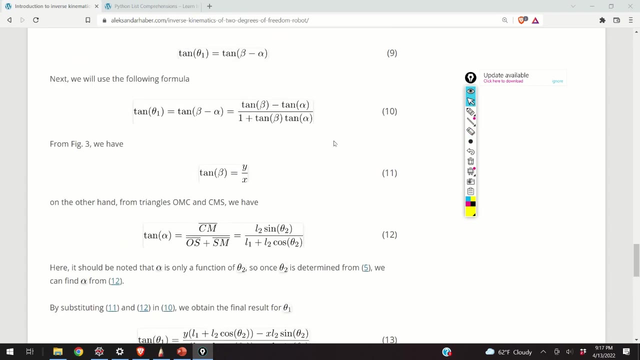 or we can express sinuses with cosinuses And we can express, for example, cm as what. There are many ways to do that. You can use tangents or cotangents or different trigonometric functions. However, here we will see that cm is L2 sin, theta 2.. 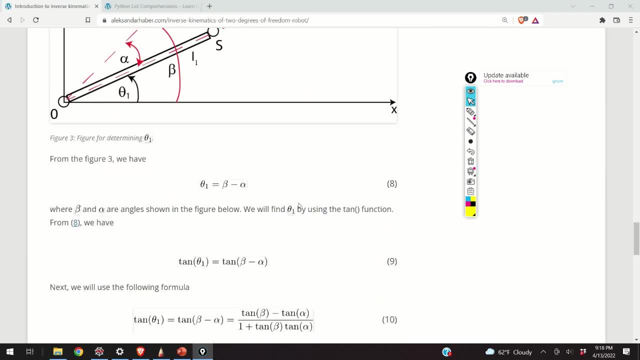 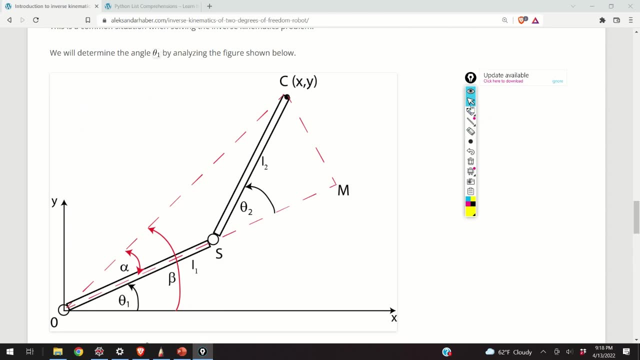 So it's L2 sin theta 2.. That's the edge And the other side of our triangle. this side over here, basically this side over here, is equal to this part. So this part plus this part, So this part over here is nothing less than L1. 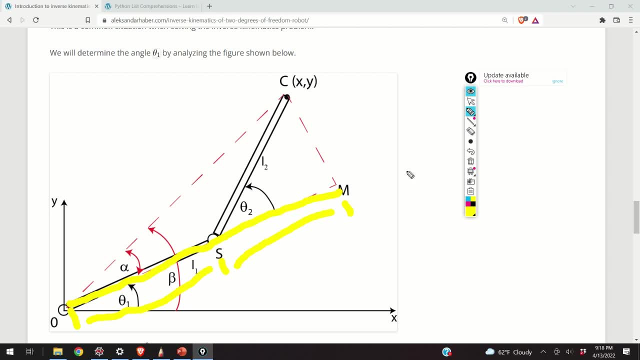 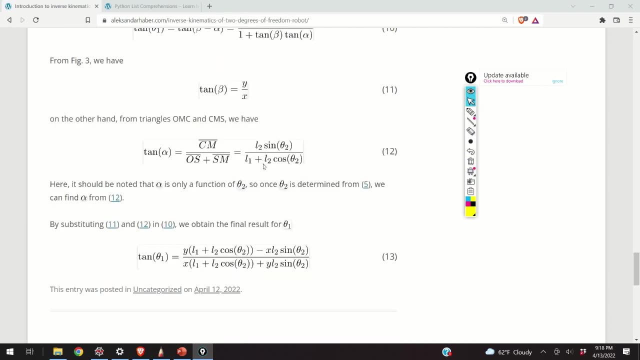 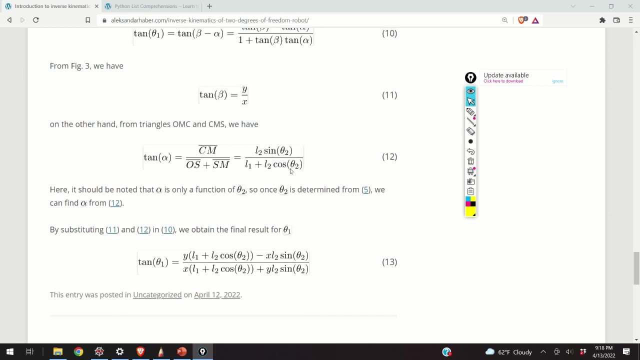 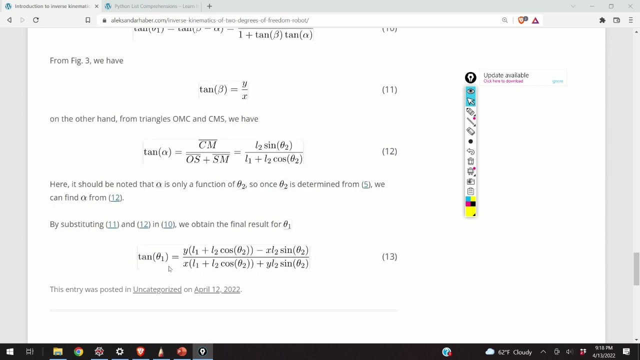 and another part is what L2 cos theta 2.. So using this and by basically substituting the values of cos theta 2 and manipulating this equation, we can obtain the tangents theta 1, actually, Or actually. let me be more precise.